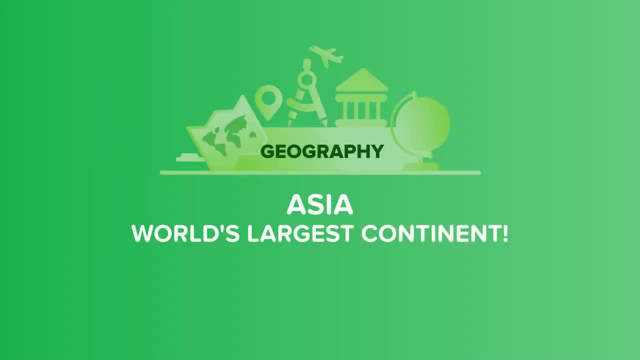 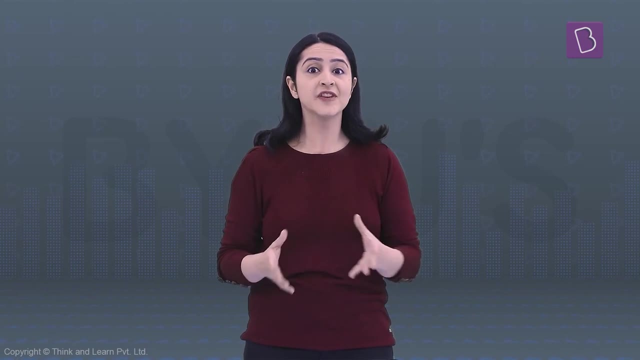 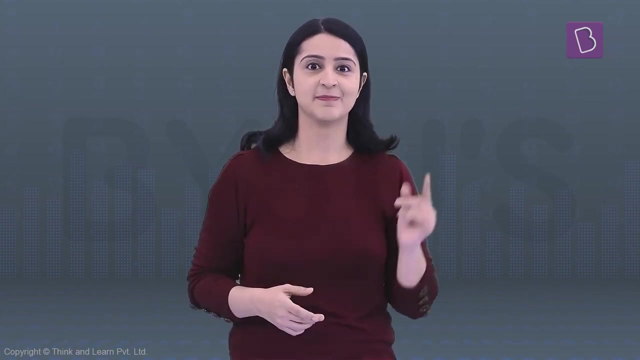 Asia is one of the most diverse continents in the world. It has a myriad of physical features: vegetation, wildlife, soils and so on. But there is one more interesting thing about Asia. It is like the bright student in your class who scores top marks in all subjects. 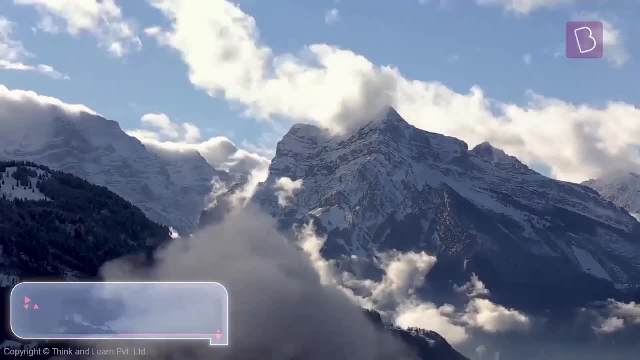 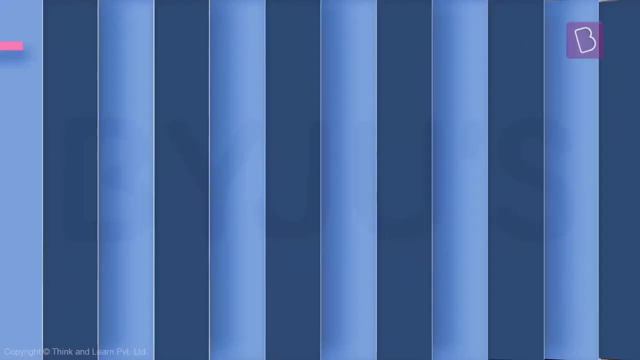 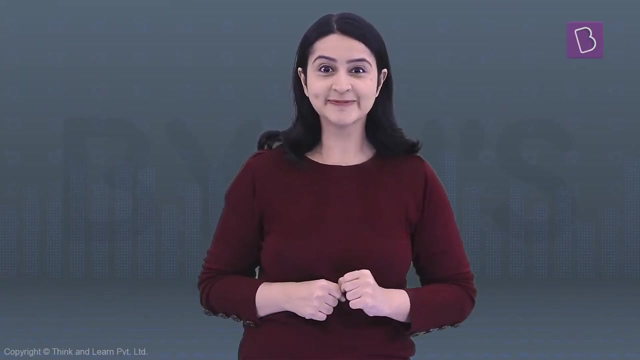 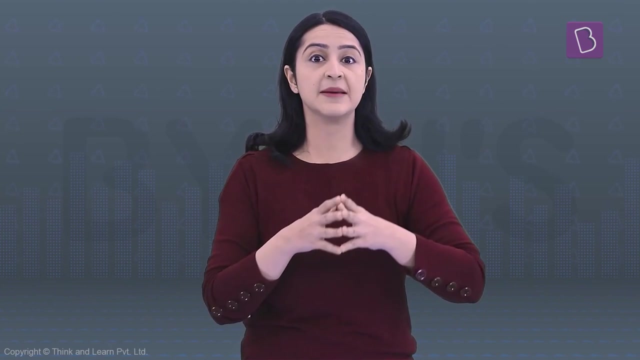 It is home to the highest peak in the world, the highest plateau in the world and the largest extent of lowlands. Other continents must be feeling jealous. Asia's diversity is not limited to just landforms. It's immensely diverse in terms of the people, languages and religions. 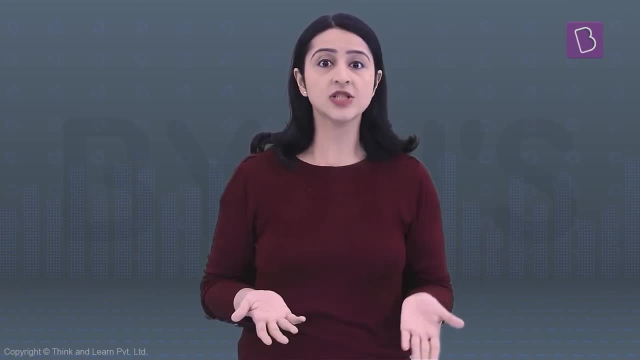 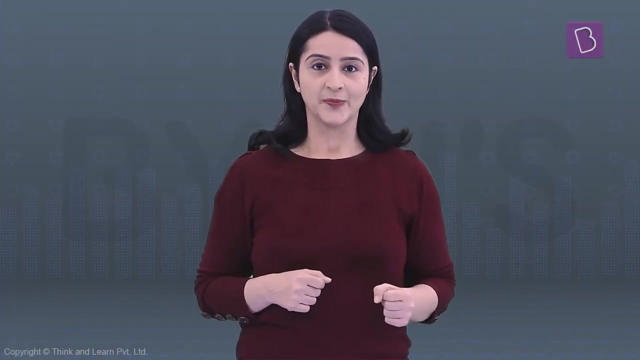 I mean, every continent has varieties of one kind or the other kind, But Asia's diversity is just mind-blowing. That's why it is known as the land of contrasts. That doesn't surprise me, though. The biggest clothing shop in your city has the widest varieties of clothes, right? 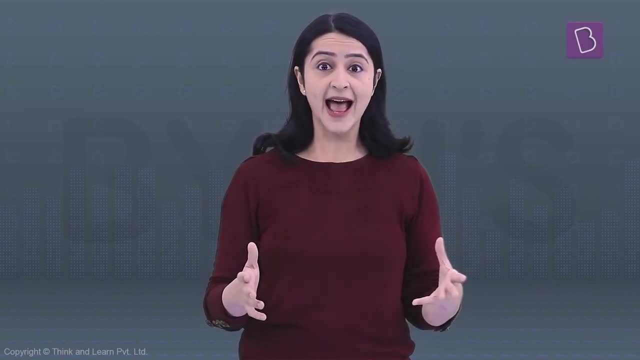 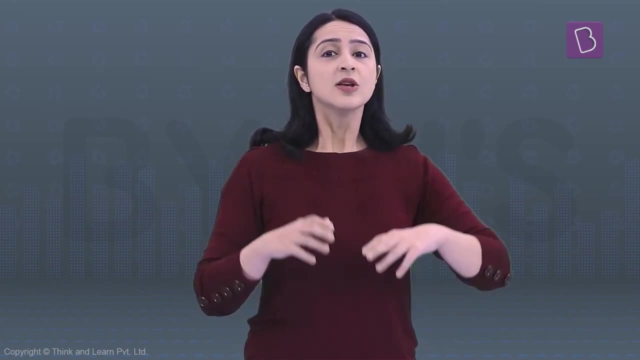 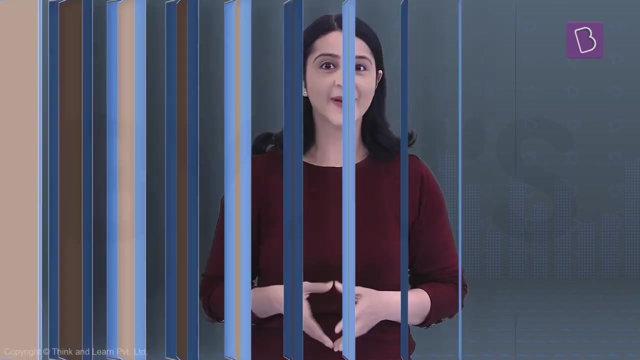 Similarly, the biggest continent of the planet has a higher chance of being the most diverse one as well. So where exactly is Asia located? Where does it lie on the globe? Alright, let us demark its location in terms of latitudes and longitudes. 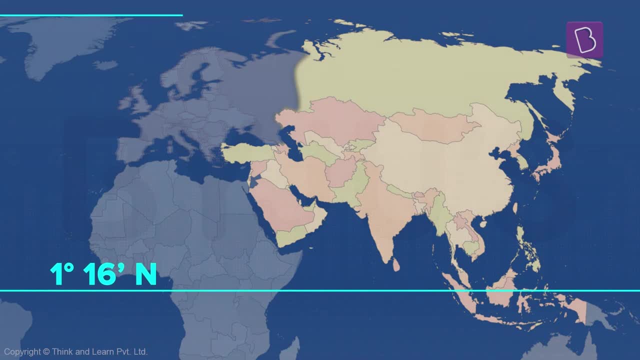 July. Asia lies between 1 degree 16 minutes north to 77 degrees 41 minute north. latitudes: 26 degrees four minutes east, 669 degrees 40 minutes east longitudes: The equator passes just south of Malaysia. Tropic of cancer passes through several countries in Asia. 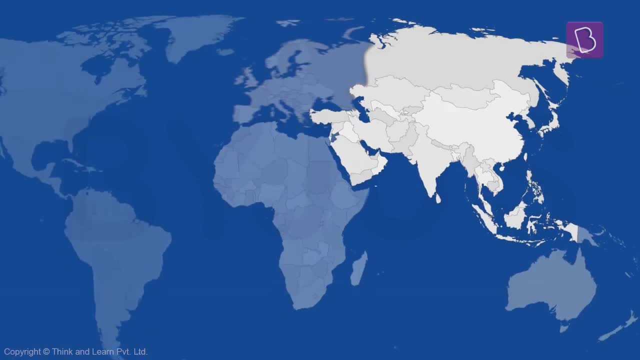 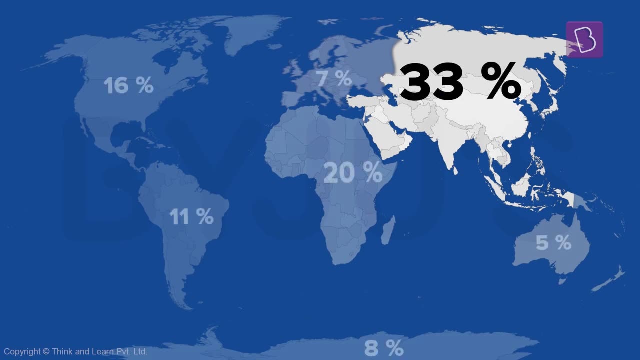 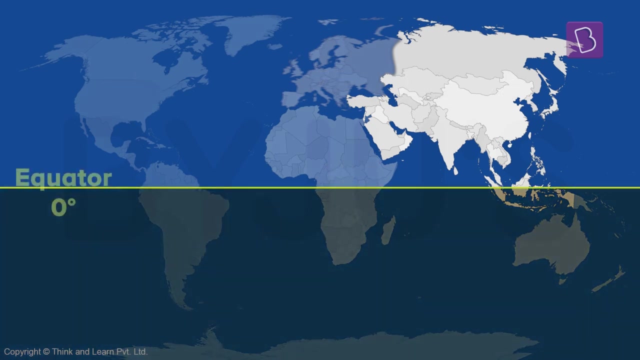 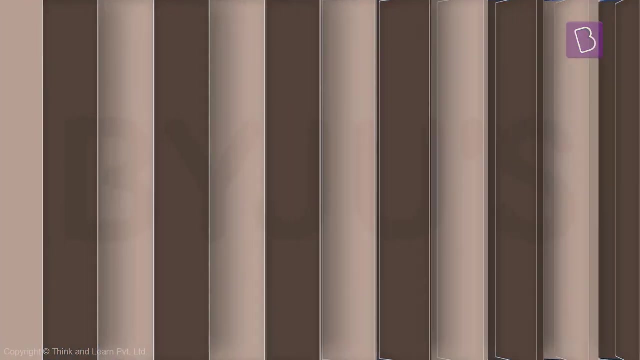 including Saudi Arabia and India. Asia is the largest continent on the planet. it covers 33 percent of the land surface of the world. It lies predominantly in the northern hemisphere. The geographical area of Asia is roughly 44 million square kilometers. Every landmass in the world is surrounded either by other landmasses or